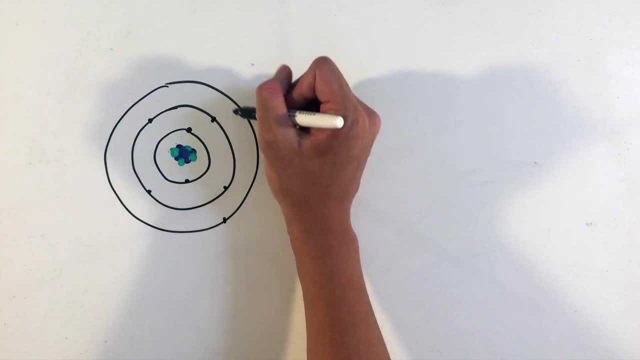 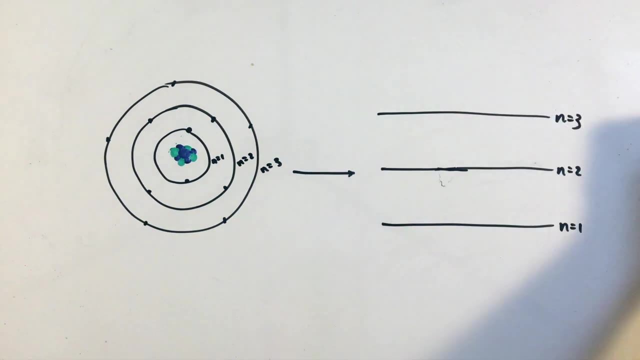 atoms are structured with a central nucleus made of neutrons and protons, with electrons that orbit the nucleus at discrete energy levels, which we'll represent through the Bohr model: different rings where electrons orbit, representing different energy levels. The main topic we'll discuss in 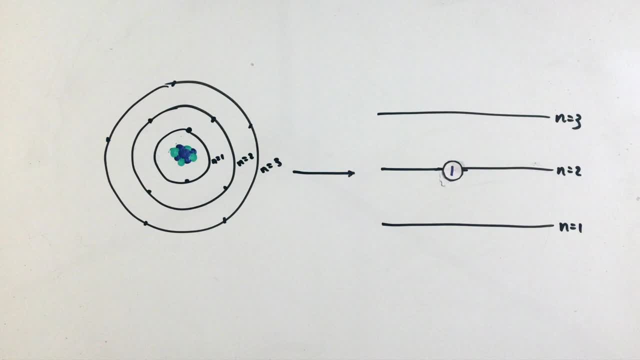 this area is when these electrons switch between different energy levels. When an energy is imparted or the atom is excited, the electrons can actually jump to higher energy levels from before and can later fall down to lower levels over time. When these electrons drop. 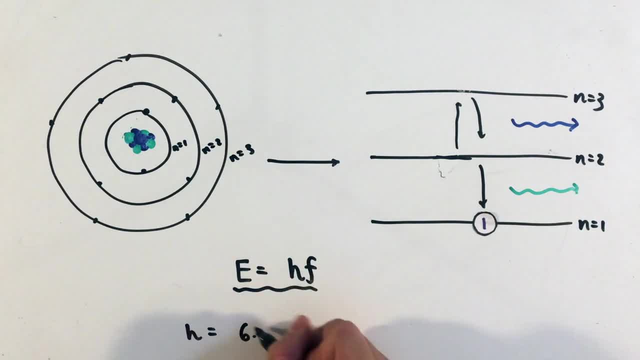 energy levels. the released energy is emitted as light or photons with the frequency given by this equation. The little letter h here represents Planck's constant, which has a value shown here. Another topic related to atomic and nuclear physics is radioactive decay. 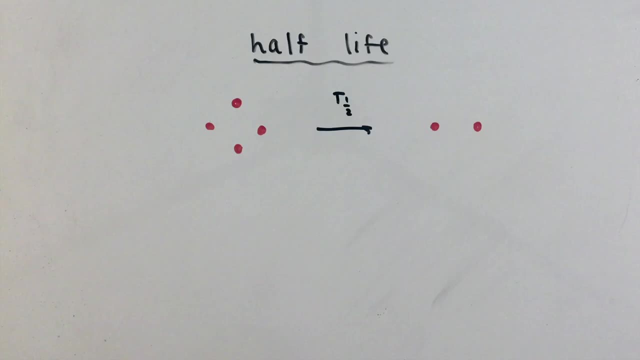 or the natural decay of certain unstable isotopes of certain elements. The time measurement used in these problems is known as the half-life, or the time it takes for a sample of some radioactive substance to decay by half. Using this information, the mathematical model that describes 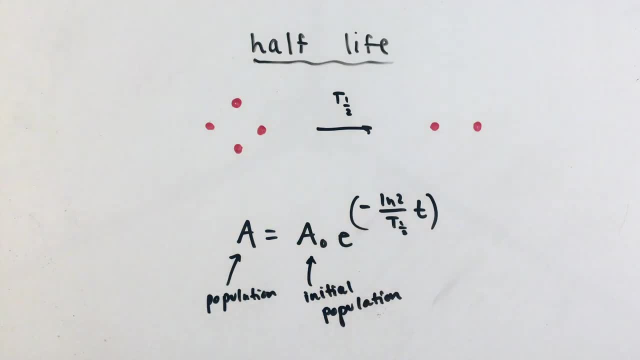 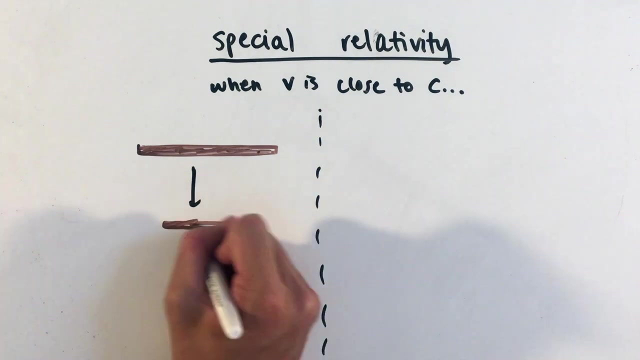 radioactive decay looks something like this, or an exponential decay based on the initial population as well as the half-life. A completely different topic that only requires a qualitative understanding for this course is special relativity. Essentially, when objects move at speeds that are near the speed of light or c, space and time are warped, Namely moving objects. 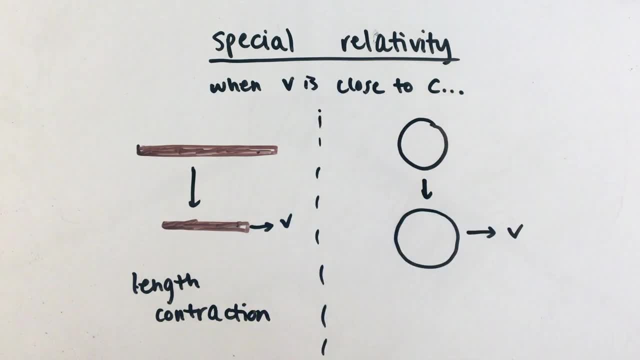 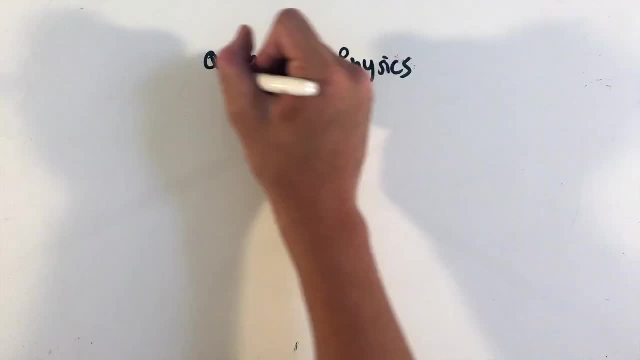 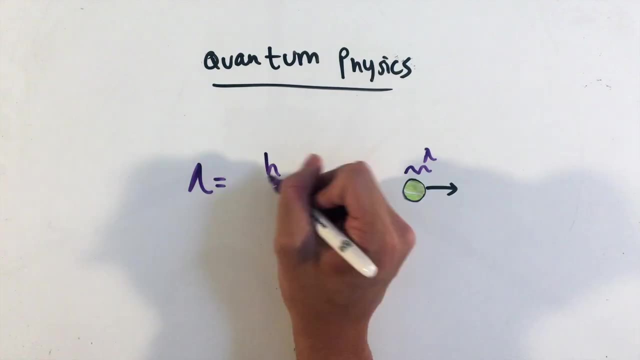 appear shorter through a phenomenon called length contraction, while moving objects experience time slower through a phenomenon known as time dilation. Another topic where our classical understanding of the world is warped is known as quantum physics. One of the most famous concepts of quantum physics is known as the de Broglie wavelength, which has the equation shown here: Essentially, any object, 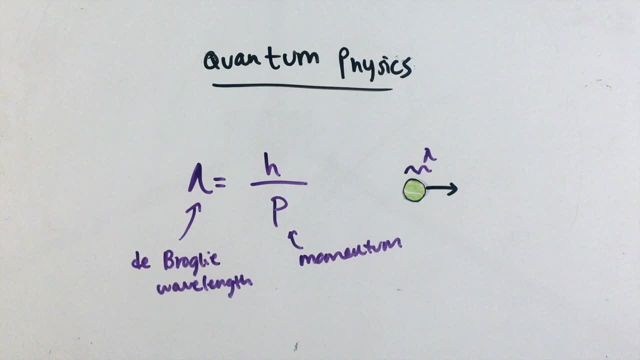 with momentum actually has a wavelength associated with it, though it'll be essentially 0 unless the object is extremely tiny, Though this leads to phenomena such as the wave-particle duality of certain objects and diffraction patterns. you'll only need to know the phenomenon. 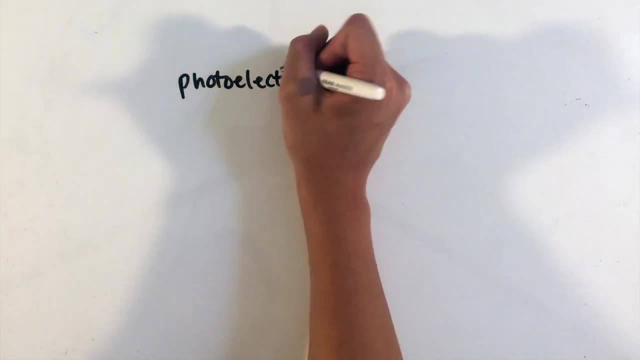 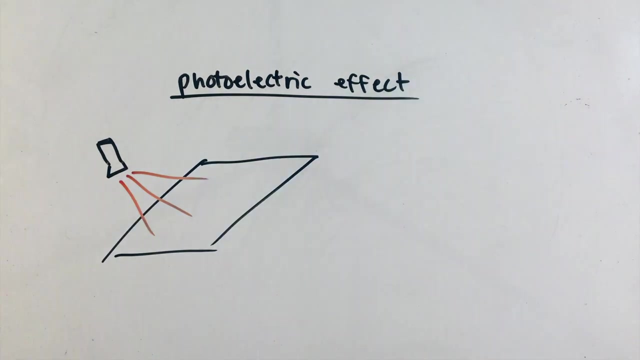 and the formula itself for your test problems. The final topic covered in this modern physics unit is called the photoelectric effect, Attributed to Albert Einstein. the photoelectric effect essentially states that light shown on materials can actually emit electrons from it. The equation: